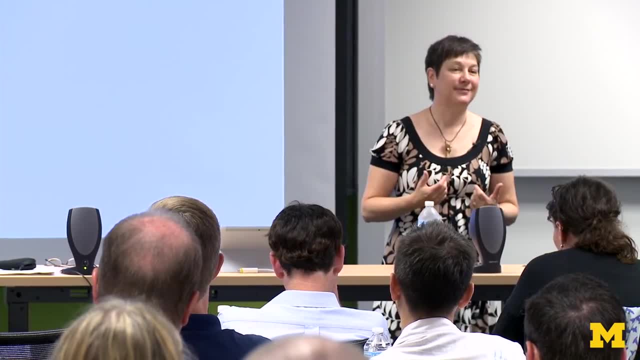 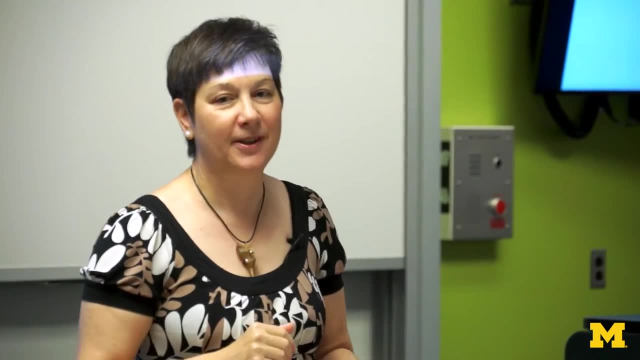 Imagine that you wake up in the middle of the night and you have a headache. So you go to your cabinet in the bathroom, you take out a bottle of pills, you take two pills, you go back to sleep. You wake up in the morning and you realize to your heart. 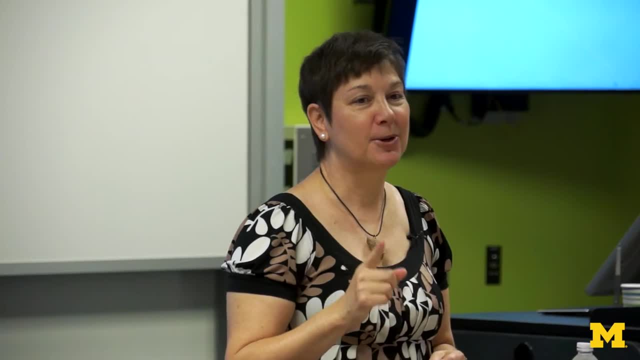 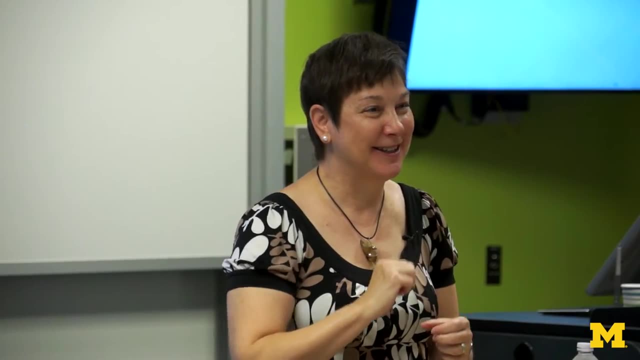 uh-oh, I had two bottles of aspirin in there, I had a bottle of poison in there And they're all the same shape, And I didn't listen to my little, you know speaking- pill bottle, So I don't know which one I took. All right, So a priori, three bottles. 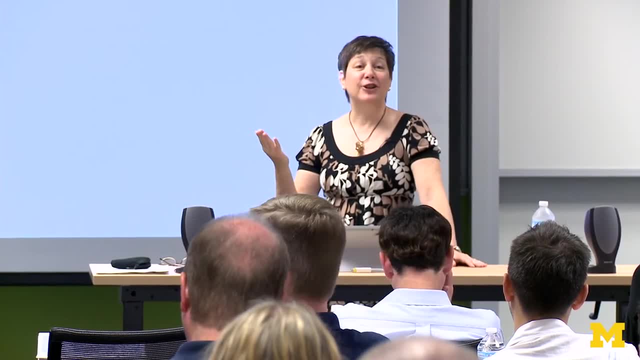 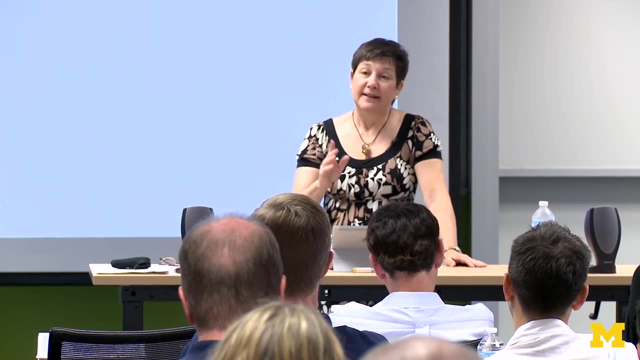 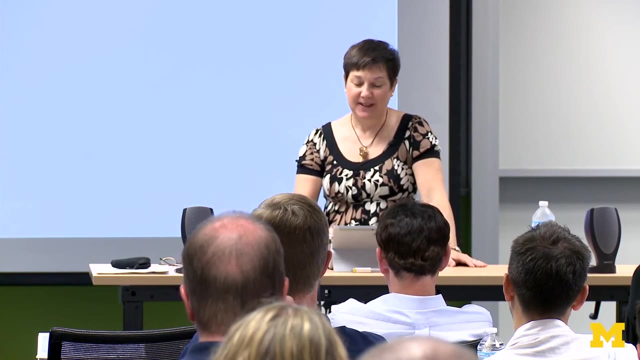 Two of them are aspirin. One of them is poison. The likelihood that you took the poison is one third. The likelihood that you took the aspirin is two thirds. Now I'm not feeling so hot And I'm thinking, okay, why am I sick? And I think, okay, if I took the poison, it's 80% likely. 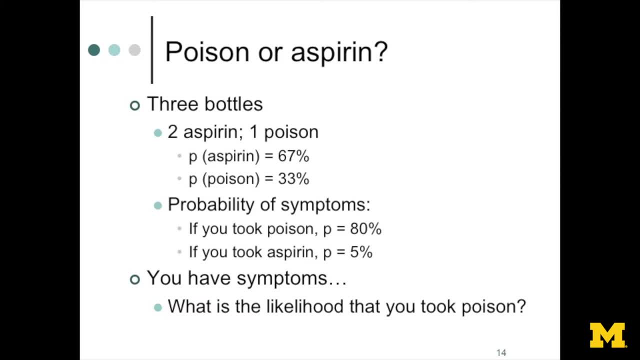 that I would have gotten sick. Took the aspirin. it's only 5% probable that I get sick, So the likelihood is the end. All of a sudden, you'll wake up. you're doing the act on a daily basis, closely to the person next to you. 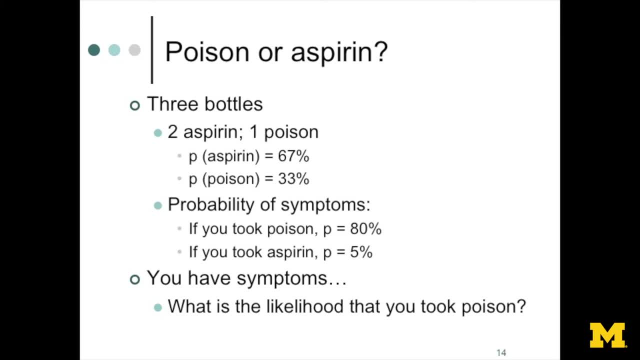 And they'll ask you: what did you do? where's the last thing you did? what did you do and why didn't you think it was appropriate? probable that I get sick? so likelihood of getting symptoms from the aspirin is 5%. the likelihood from the poison is 80%. so the question is, now that you have 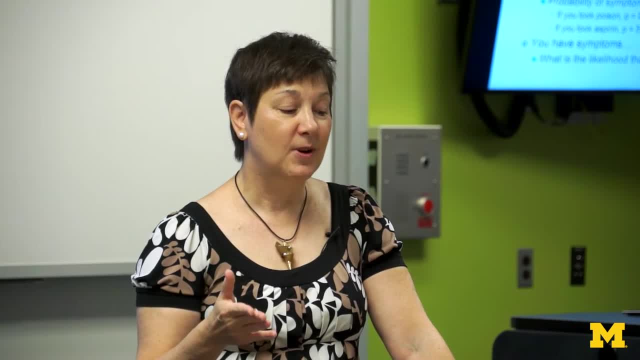 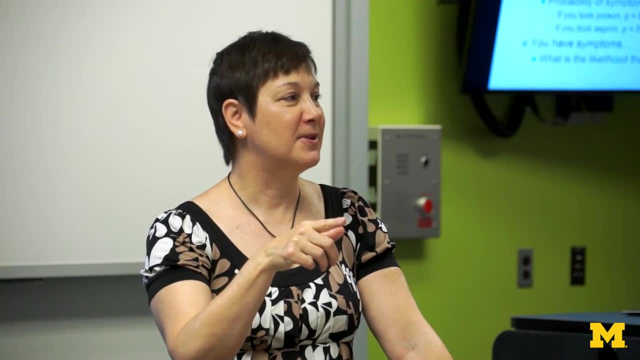 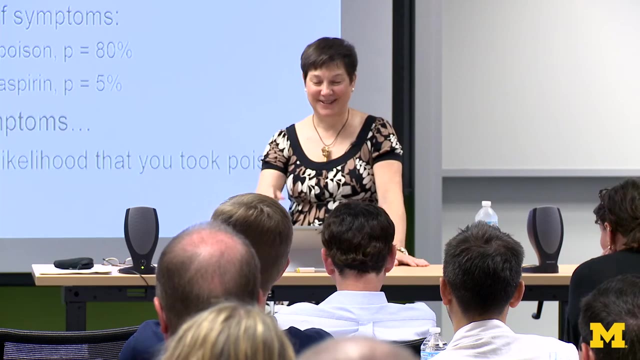 symptoms. you're not feeling so hot. what's the likelihood that you took the poison? 33%? I heard 50% somewhere. anybody else want to guess? all right, we've got numbers all over the place, all right? well, let's think about it. how could you? 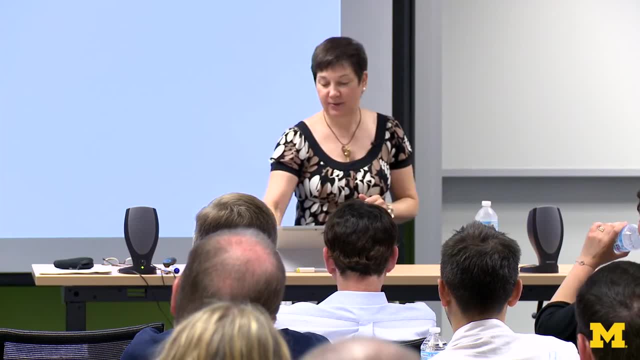 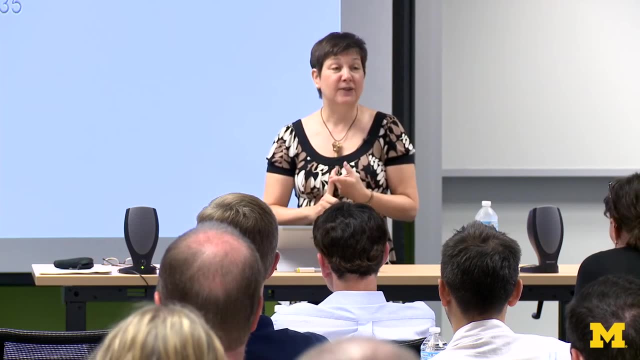 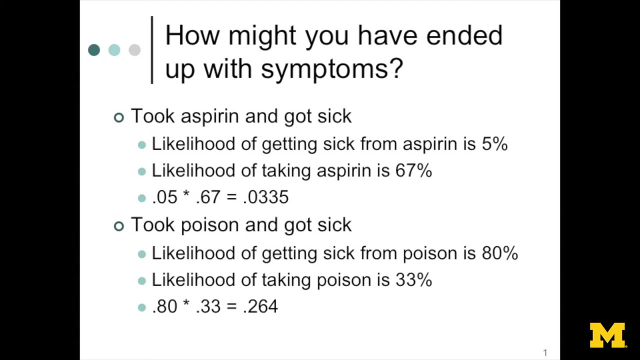 have ended up with symptoms. what are the ways in which you could have gotten sick? right, one of the ways is you took the aspirin and you got sick. and if we do, the probabilities- the likelihood of getting sick from the aspirin- was only 5%, even though the likelihood of taking the aspirin was 2 thirds, or 67%. so if we 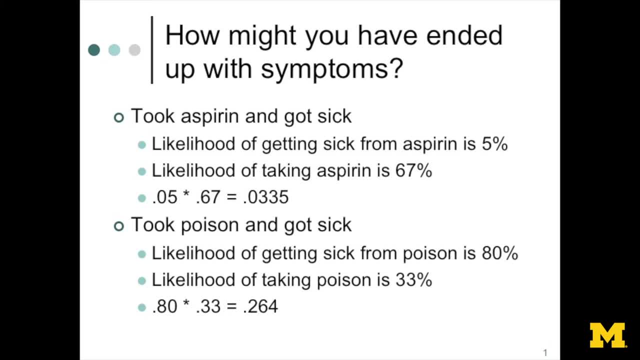 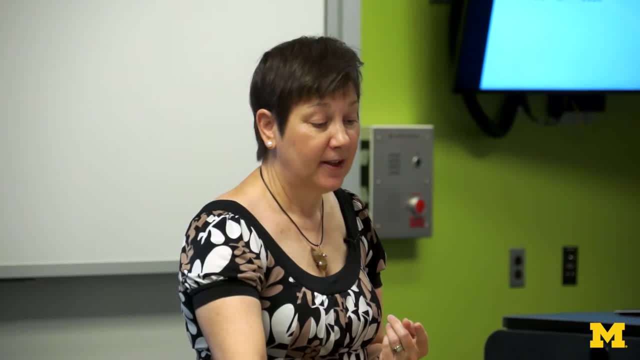 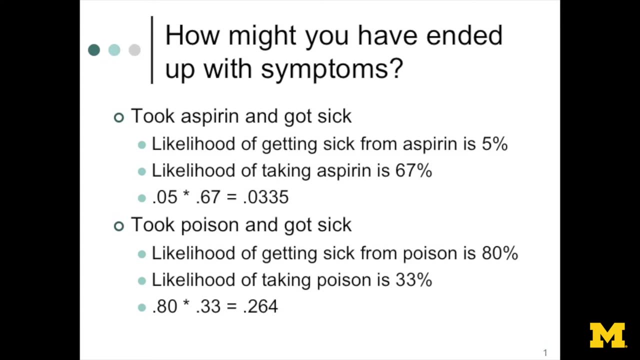 do the actual math, which I know you're not doing in your head. 5% times 67% is 3%. okay, 3% likelihood that you would get sick- okay. on the other hand, if you took the poison and you got sick, likelihood of getting sick from the poison is 80%. the 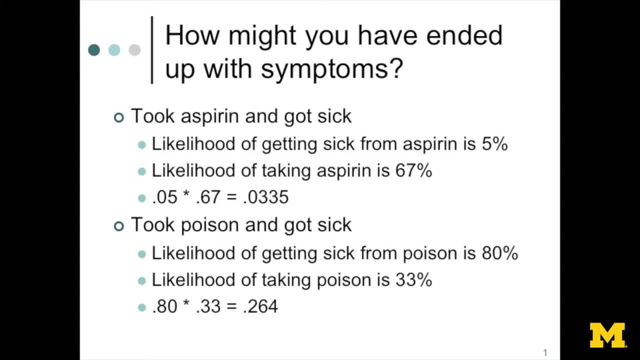 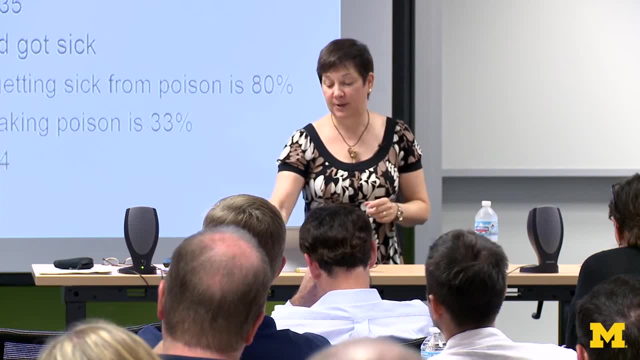 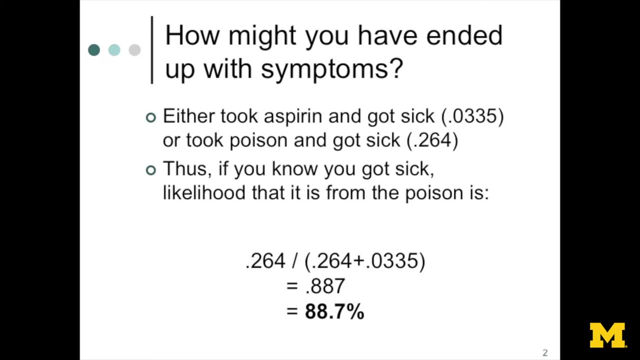 likelihood of taking the poison only 33%, but that is 26% all right. so now, if you think about the total number of ways in which you could have had the symptoms, you could have either taken the aspirin and gotten sick, which is 3% roughly, or 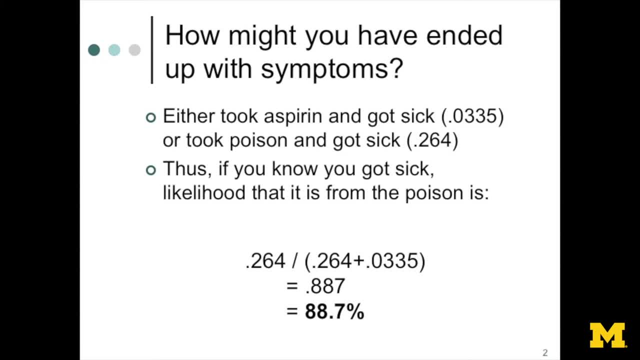 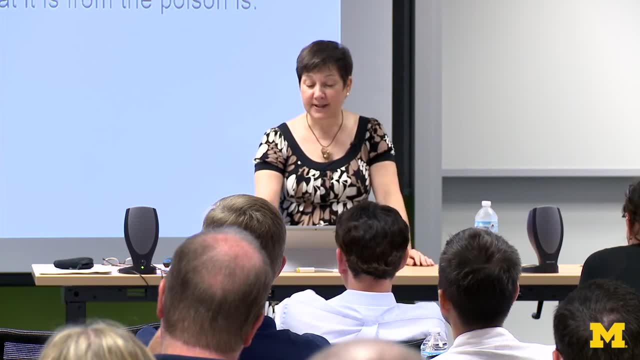 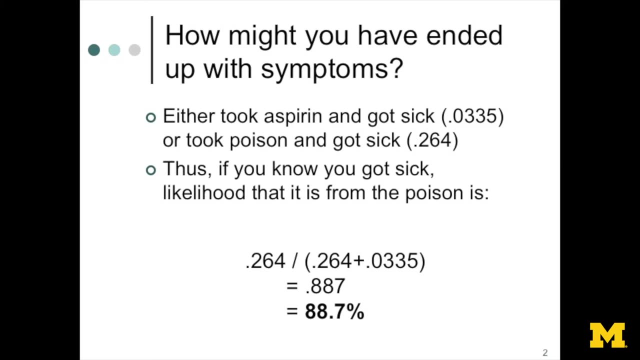 you could have taken the fashion and gotten sick from the aspirin, taken the poison and gotten sick, which is 26% likely. So if you know you got sick, you know that you got sick. the likelihood that it came from the poison is 88.7%, or almost 89% right. 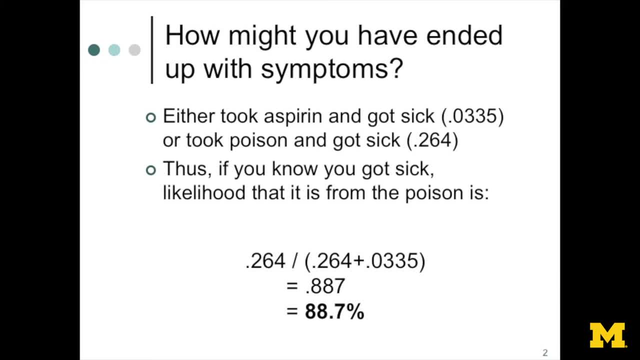 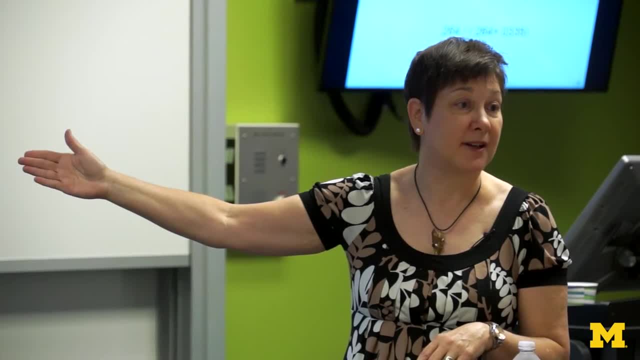 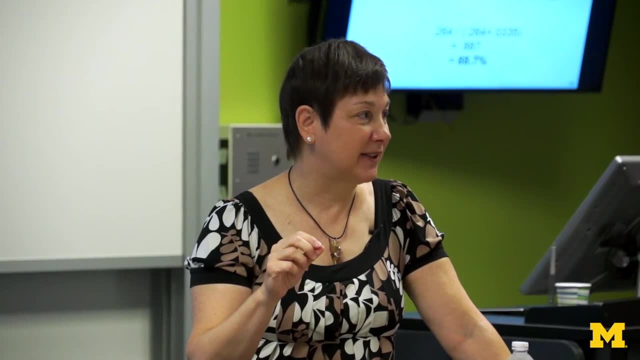 That is, the .264, is the likelihood that you took the poison and got sick over the total ways you could have gotten sick, which is either by taking the aspirin or by taking the poison. So now that you know that you had symptoms, right, the likelihood has increased dramatically. 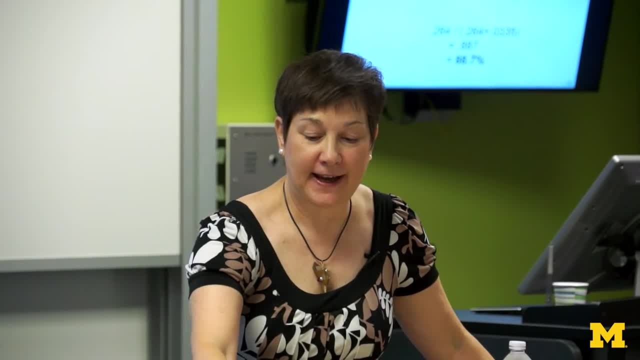 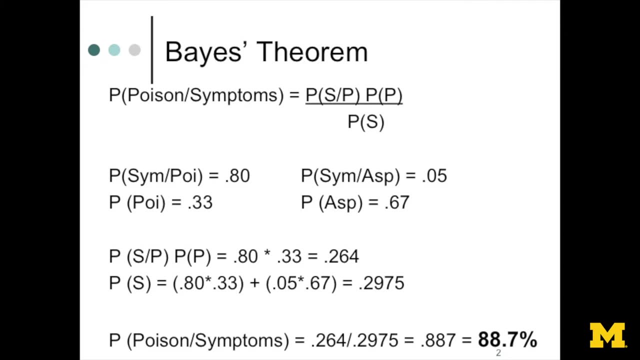 that you took the poison right And in fact, this is something called Bayes' theorem. That's the math And there will be a handout that I'll give you at the end that has this math on it, so you can check my math. 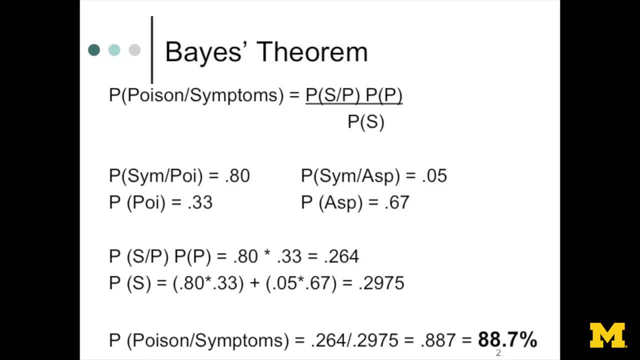 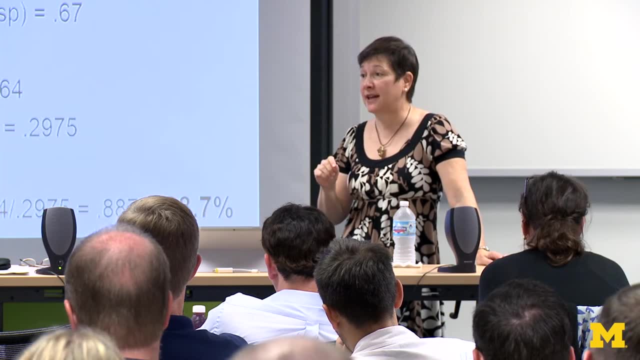 But believe me, this is correct. The likelihood of having taken the poison has increased dramatically because you have symptoms and because it's so unlikely that you would have gotten sick Had you taken the aspirin. So this demonstrates the fixation or anchoring bias. 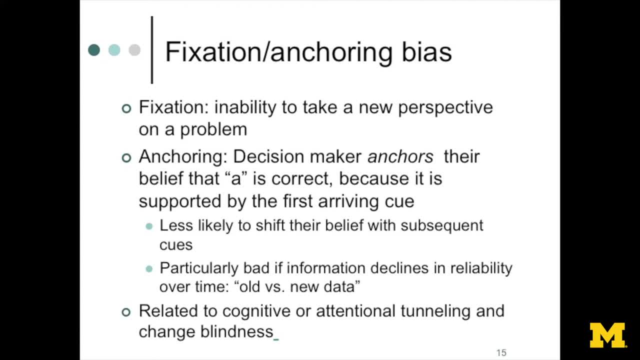 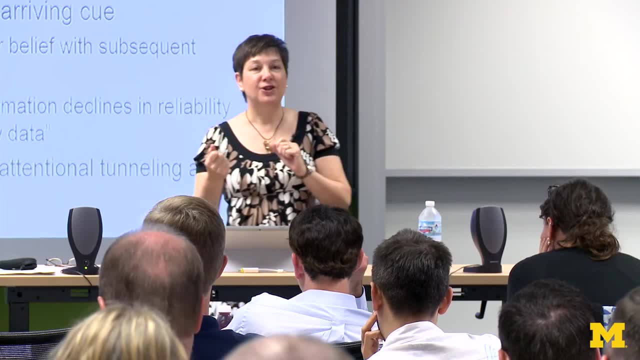 That is, we tend to kind of fixate, We get fixed right. The likelihood ahead of time is one-third. So we think, well, it's still one-third, But we have new information. That new information is that we're now sick. 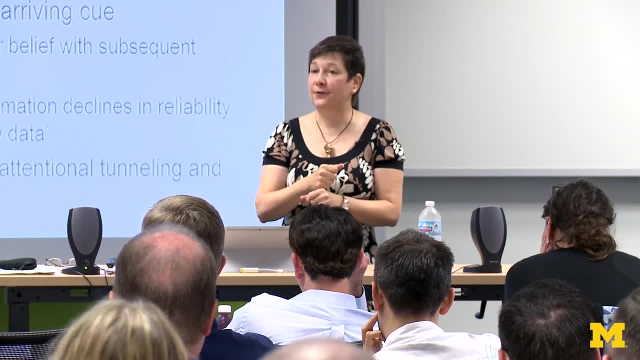 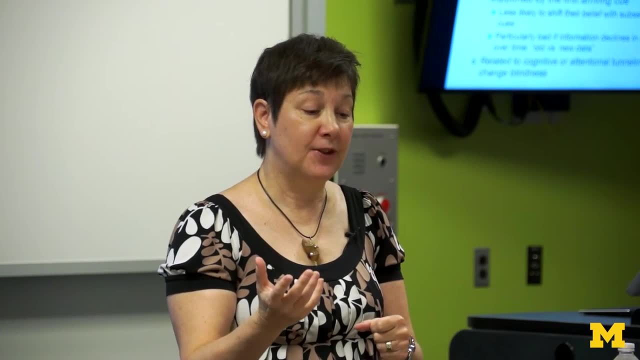 And we don't use that information to adjust sufficiently. We've kind of anchored ourselves in that one-third probability And we don't adjust upward, Upward sufficiently. Okay, Now, this is particularly a problem if you are getting a display that gives you updates. 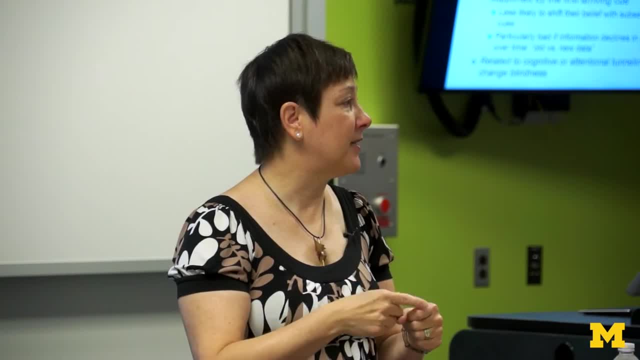 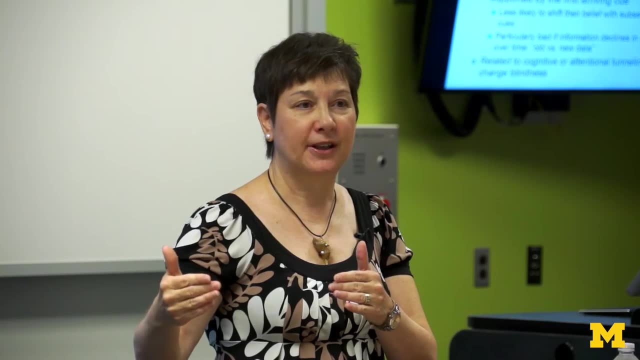 of information Right? So you've made a diagnosis of the situation and now you get an update and another update and another update. You need to recognize that people are not always updating sufficiently, because that first piece of information in is going to create that anchor. 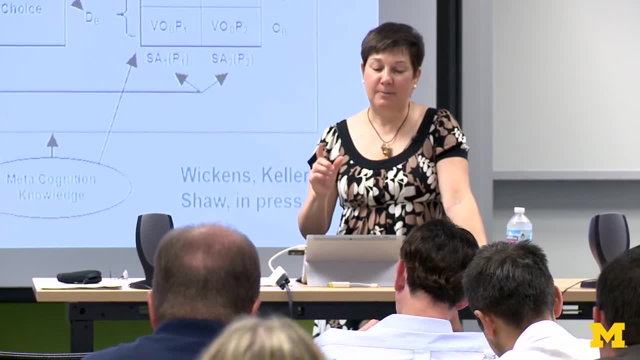 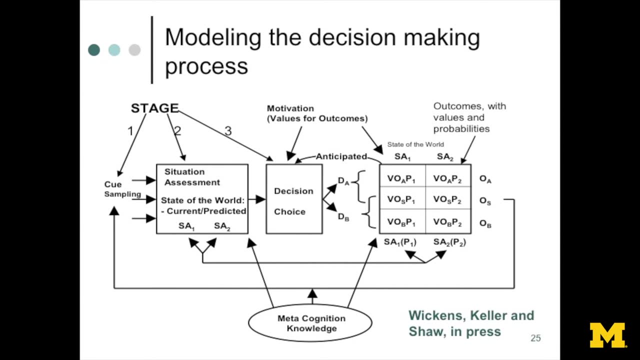 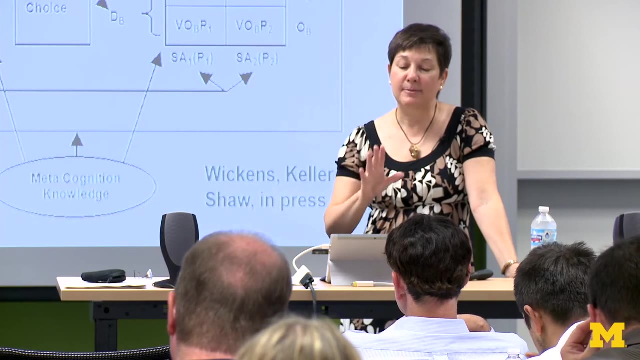 Okay, I want to talk fairly briefly about a very complicated model that Chris Wickens, Keller and Shaw have put together to talk about how we go about making decisions. It has a lot of probabilities and things in it And it's not. I'm not interested so much in getting you to understand every little nuance. 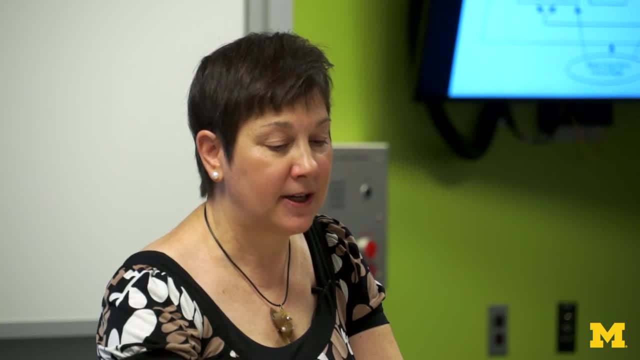 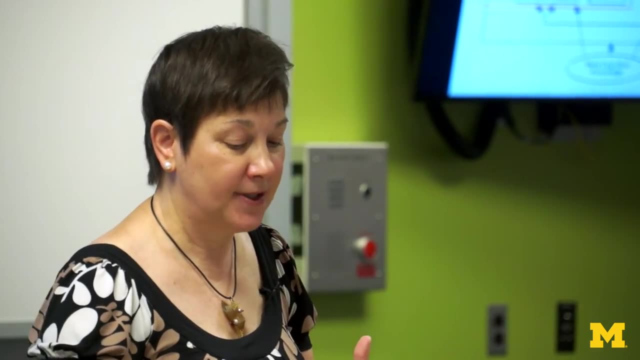 of the model. What I do want you to understand is that it's based on this notion that we have. we're processing information, Right. So there's basically three stages. There's Q sampling, which is just the piece of the information model we talked about yesterday. 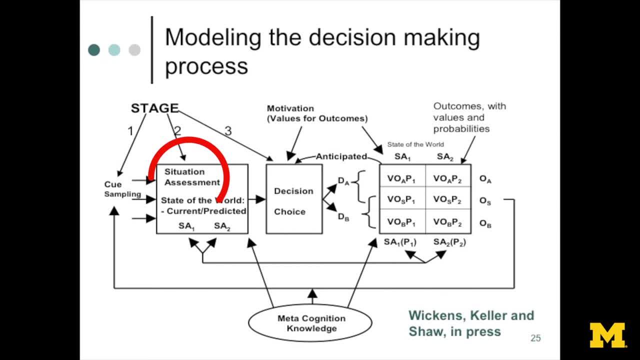 where you're taking information in from the world, right. There's then the situation assessment, the comprehension piece. There's then the decision choice- right, Making a choice about what action to take, And then each of those decisions that you could make have consequences shooting down. 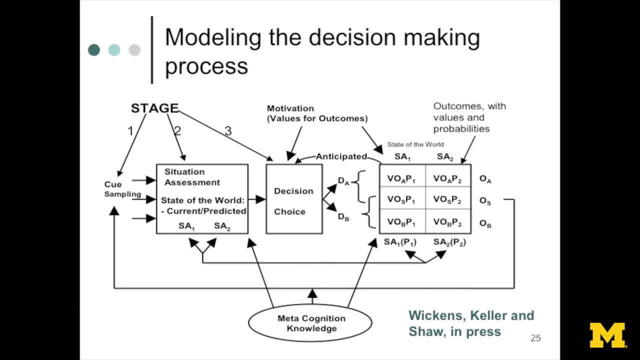 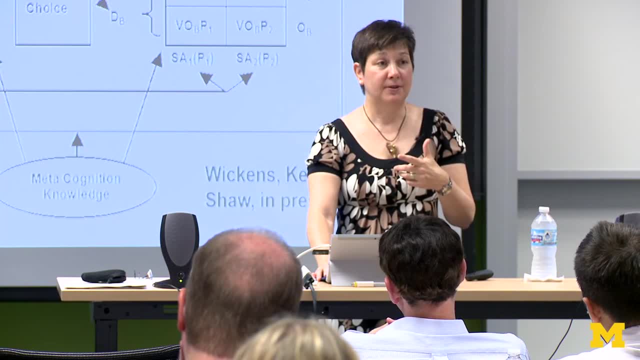 the plane, not shooting down the plane, And that leads to some outcome. Now the outcome is going to depend on the actual state of the world, Right? So if the state of the world is that it is a hostile threat, there'll be one outcome. 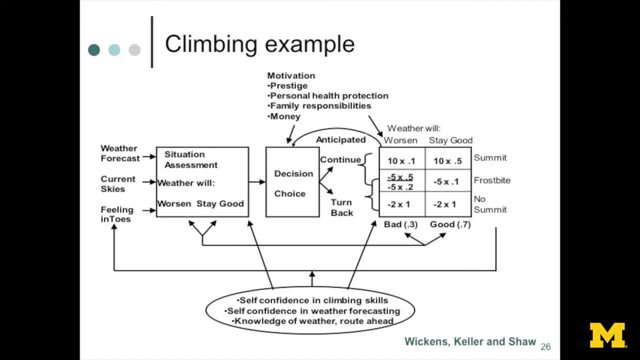 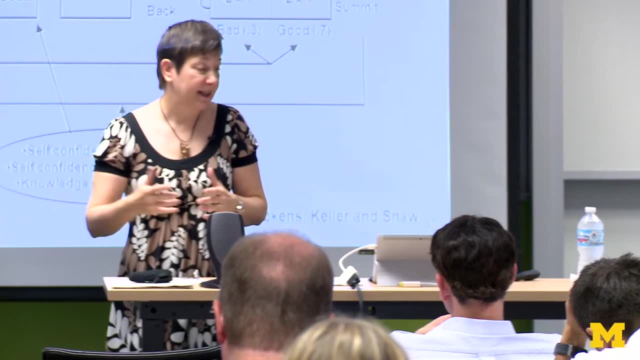 If it's not hostile, there's another one. So let me talk about this in a particular example, which will make it clearer. Imagine you're a mountain climber and you're up on the mountain And you start and in the middle of the day we have these cues that are out there. 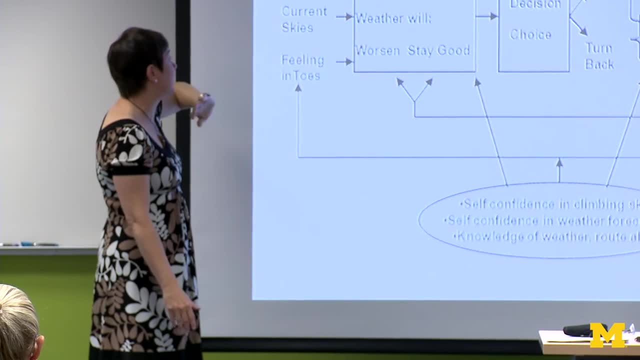 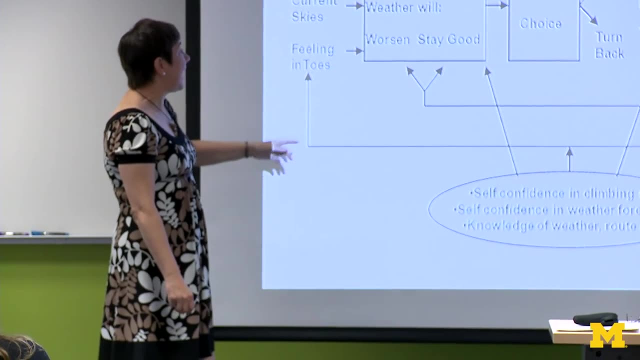 We have the weather forecast right. We all know to look at the forecast to see what the weather's going to be like. We have the current skies and we have some feeling in our toes, Or lack of feeling in our toes, because it's cold- and we're sitting there with some assessment about whether 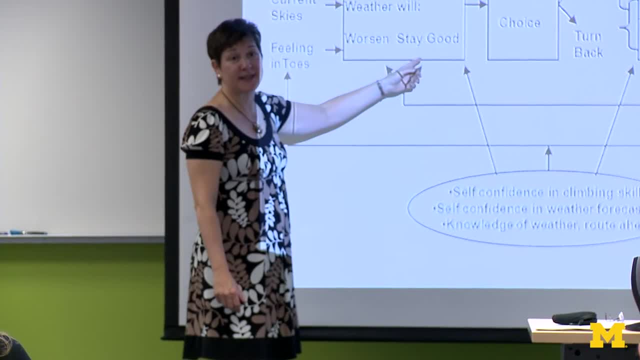 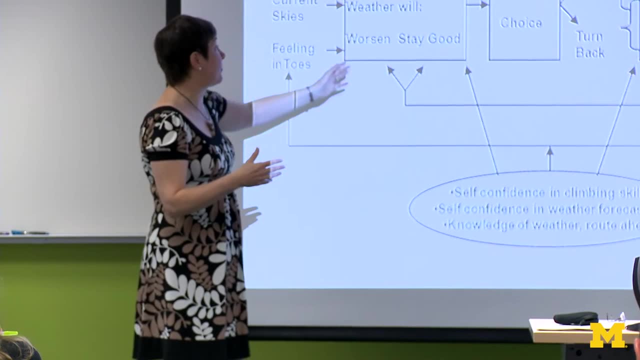 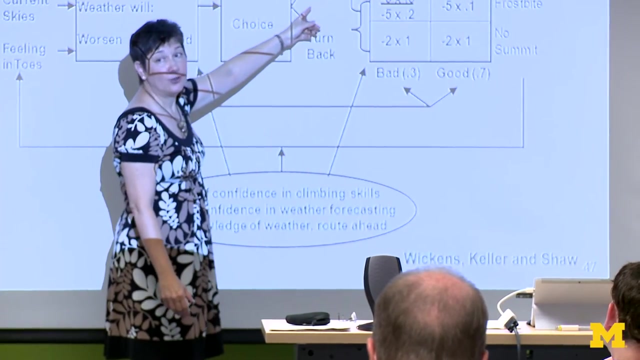 the weather is going to get worse or that's going to stay as good as it currently is. so you're on the mountain, you have some weather going and you have this choice between whether the weather is going to worsen or stay. stay good. now you have a choice. should you continue climbing or should you go back right now? 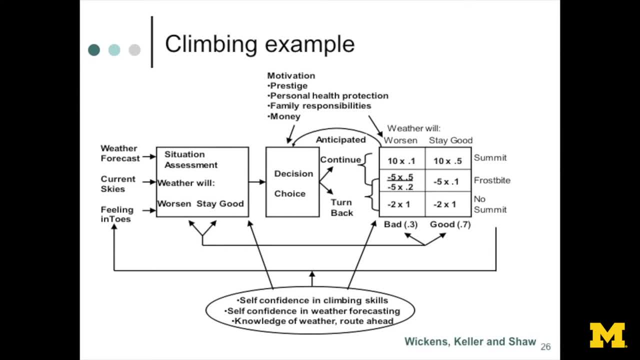 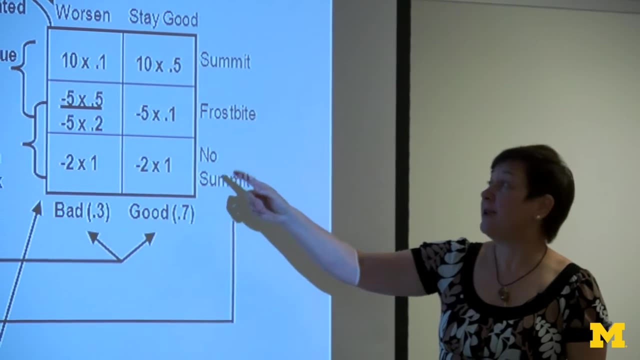 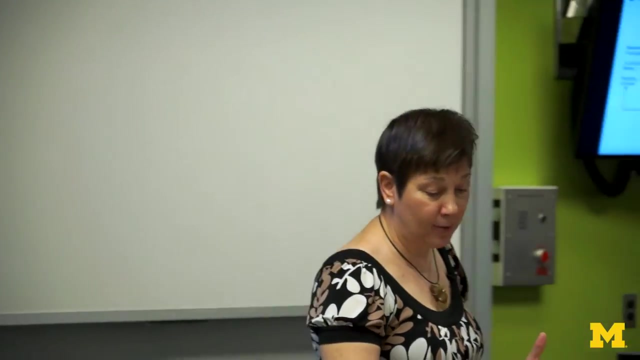 if you decide to continue, there are two things that might happen. you could reach the summit and you might get frostbite- okay. if you decide to turn back, you certainly are not going to summit. you're not going to make it to the top. you might still get frostbite. okay, and that's all going to be a function of 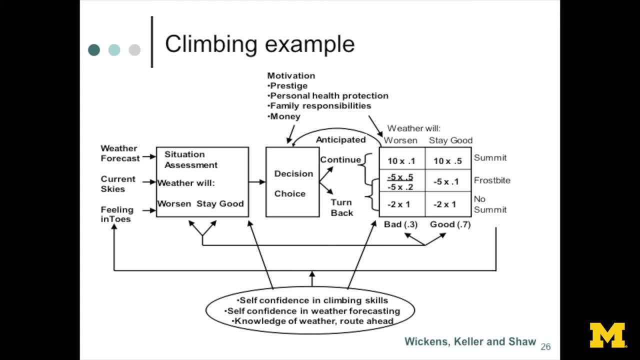 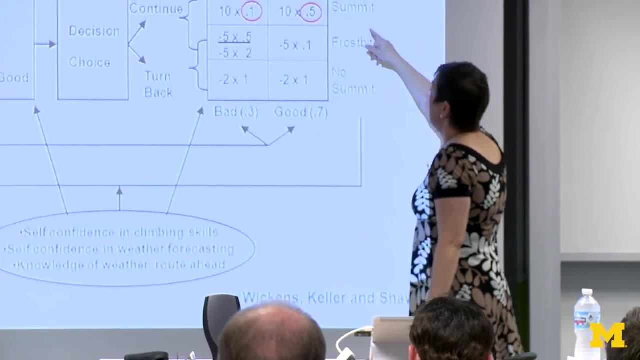 what actually happens with the weather. so we start with our forecast. we have our choices here. we continue to go back and we have these options now. if the weather worsens, the likelihood that you summit is going to change right. so if the weather gets worse, there's a smaller probability than if the weather 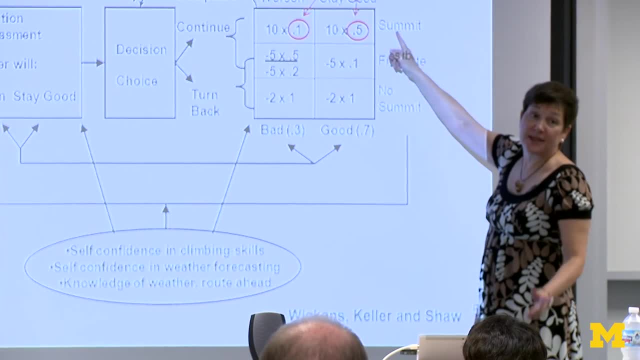 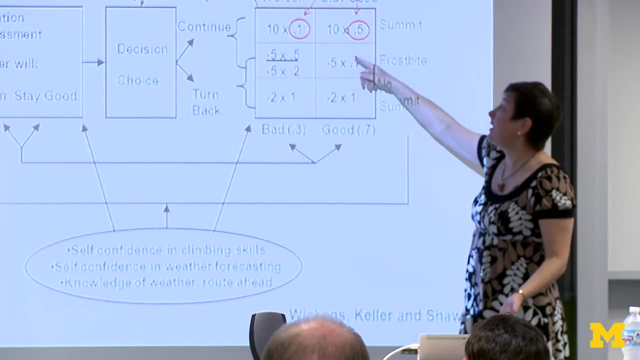 stays good that you're going to make it to the top right. so notice that, even if the weather is really good, you may or may not actually make it to the summit right, because there are other factors that influence this, but this is going to be the probability that you actually reach the 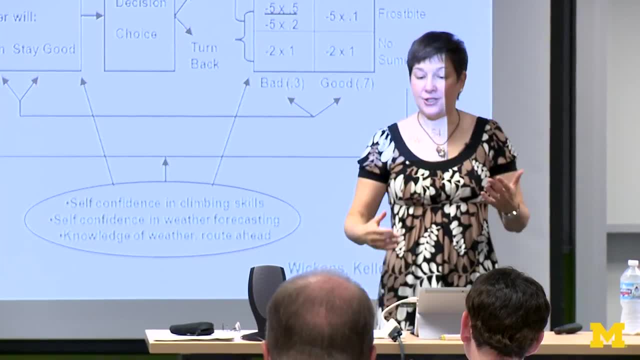 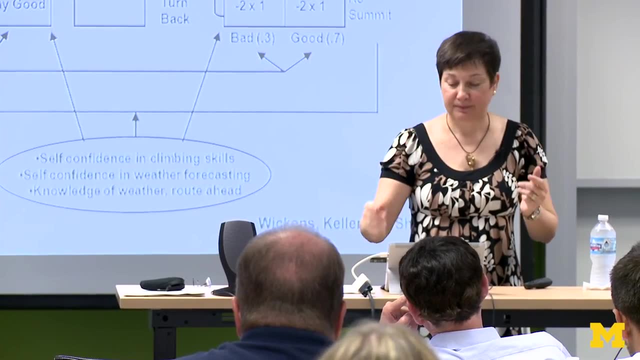 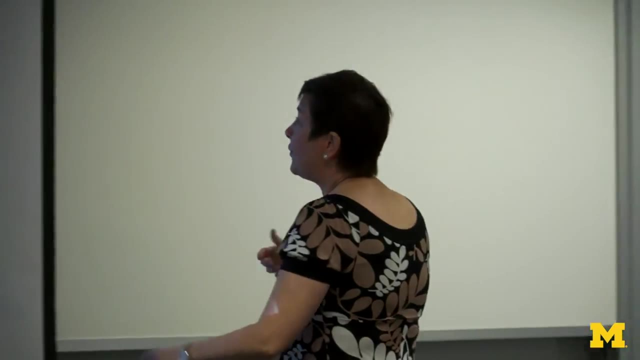 summit. this here is going to be the value that you attach to summiting, right? so it's a really positive. 10 is a positive value. you want to get to the summit. you can do the same thing for frostbite. so if you continue on, you don't like getting frostbite in any case, right-. 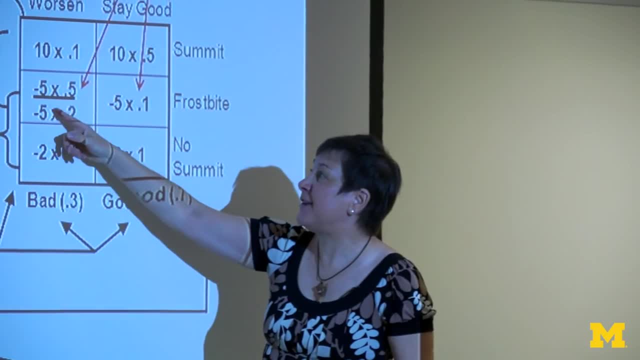 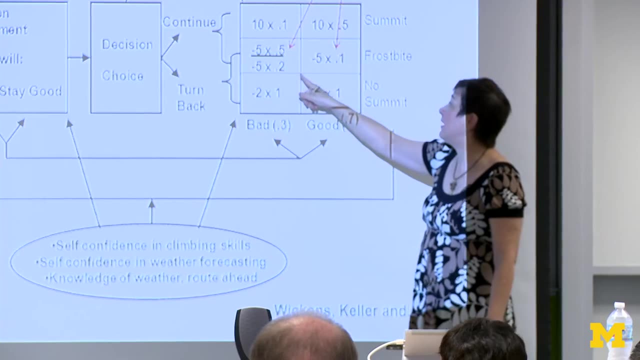 not a very pleasant thing. so negative 5 and if you continue on and the weather gets worse, there's a higher probability of you getting frostbite than if the weather. and if you go, then if you go back and over here, the likelihood is less that you'll get frostbite. if the 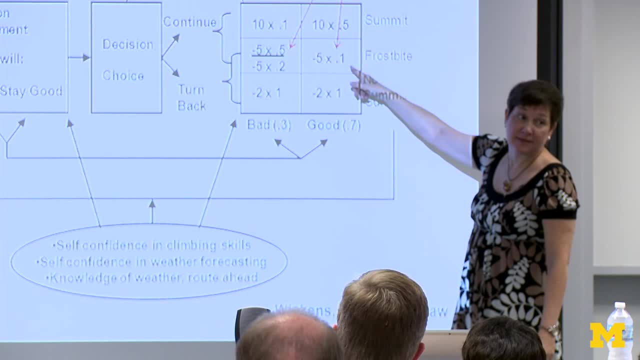 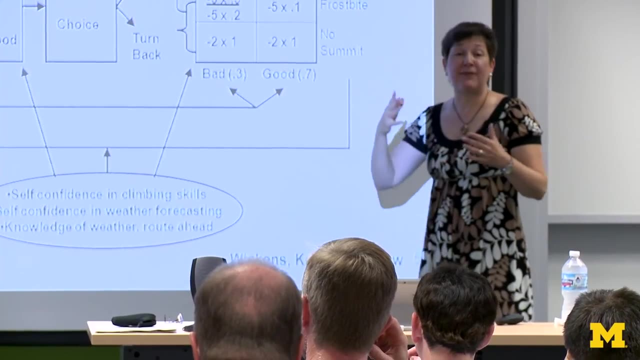 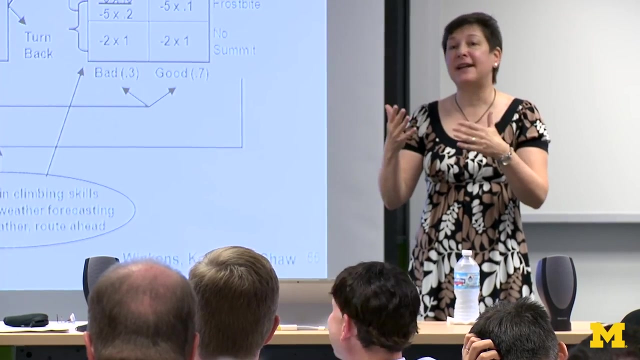 weather stays good. right, that makes sense. yes, yes, I've made them up. I mean, we don't know what they really are, but and in fact people don't really know them either, right on a scale of one, right one to ten. so the idea is: you know, 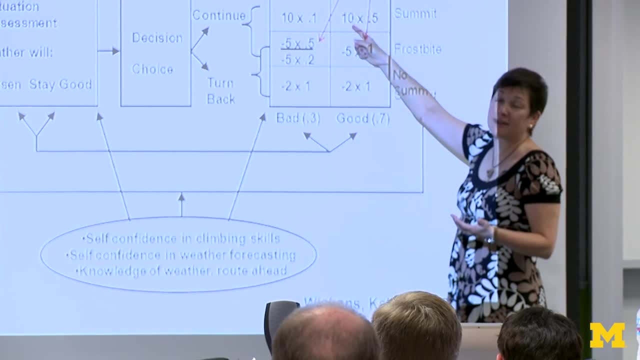 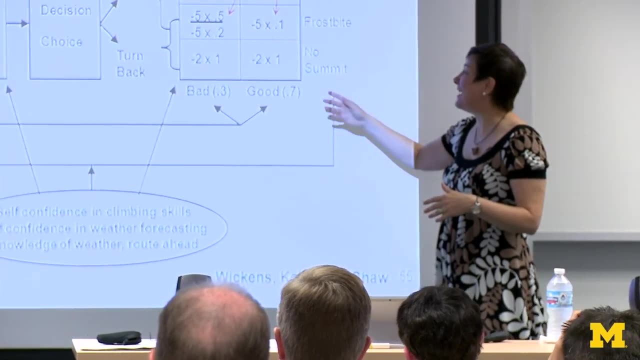 it's it. there's much more positive value associated with making it to the summit than turning back and not summiting. if you're gonna die, right, so you have this choice here. and- and here's the probability of one, we know for sure, right, if you turn back, you're not going to make it to the summit, so you don't. 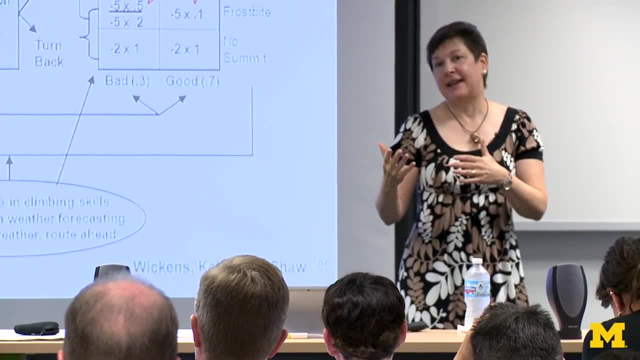 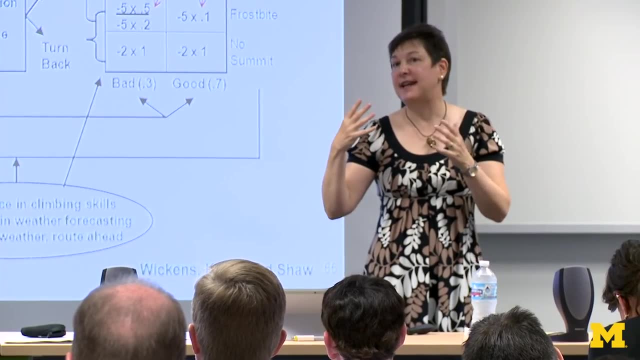 need a lot of probability to know that it's negative, that if you don't make it- and you're certainly not going to make it if you turn around, on the other hand, you're just kind of guessing. we're not saying that these numbers really exist in your head because, remember, we don't 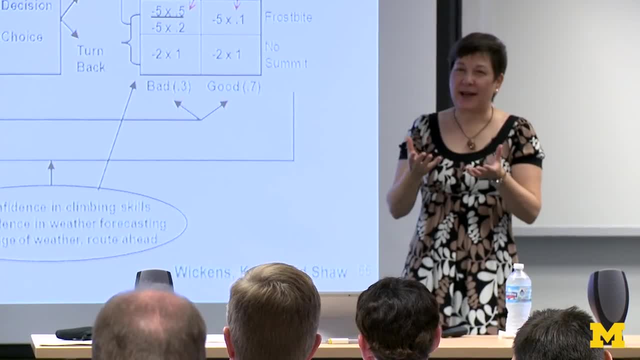 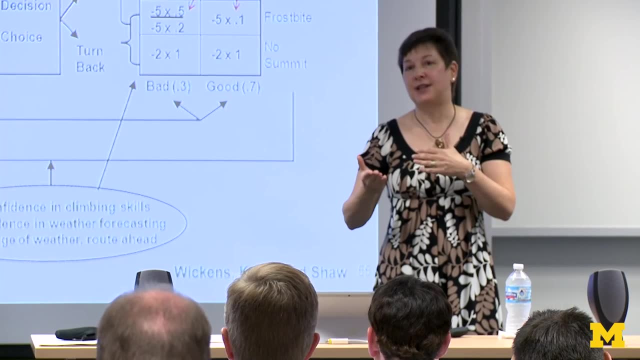 really believe people are good at probability. but you have these feelings right. you have this notion that you know for sure that it's more likely you're going to get frostbite if you continue and if the weather gets worse. so you may not know the exact amount and you're going to rely on your guide to tell you. 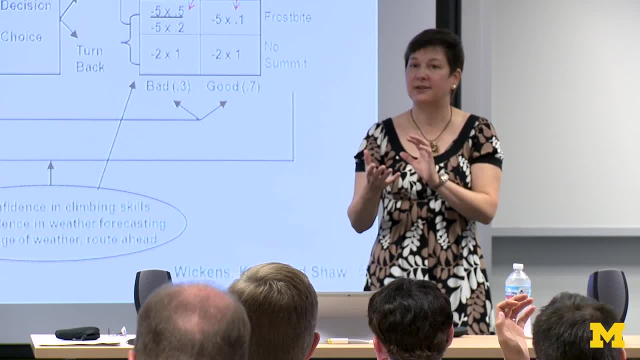 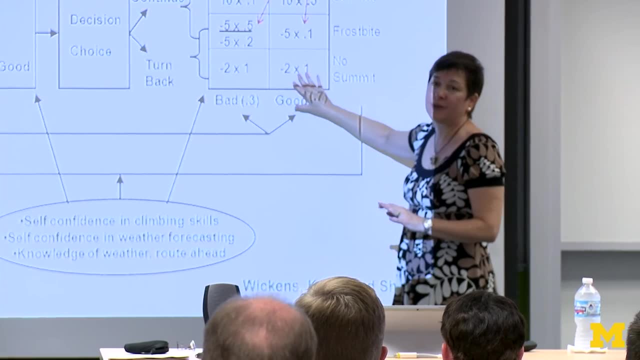 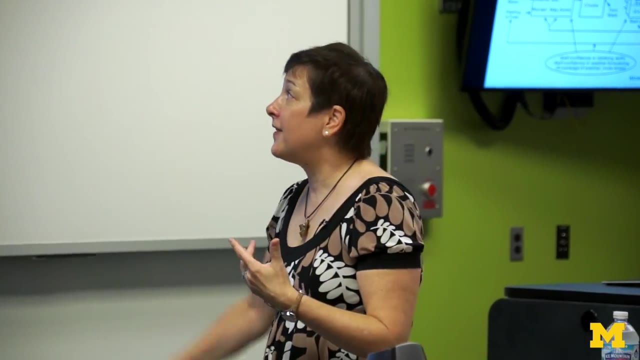 some information, because they may have more experience, and where that comes from is not clear. the bigger point here is that this is the information processing piece of making the decision. but now there are factors that go into the decision you make, but there are other things that matter, right? so motivation, prestige, you know what's going to happen if you go. 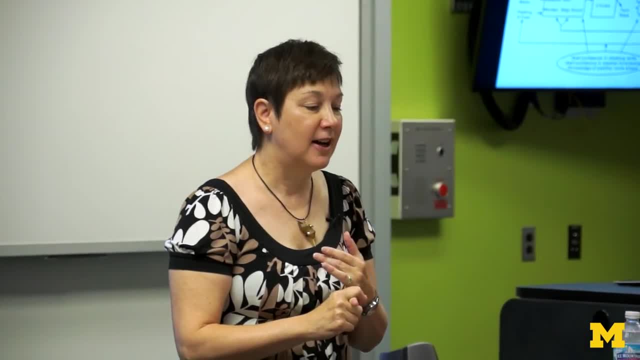 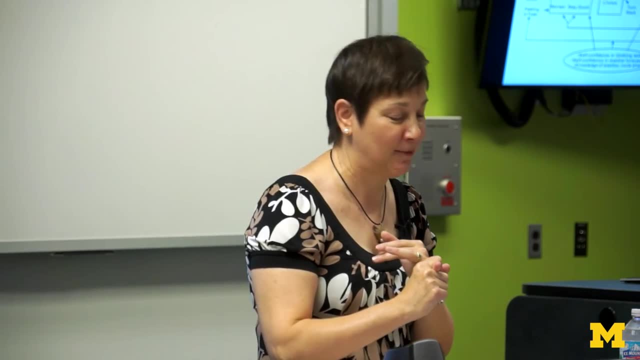 home and you didn't make it. are you going to feel bad? what your wife going to say if you didn't turn around? well, if you didn't turn around, you get killed. you're not going to know what your wife had to say, but you might have a pretty. 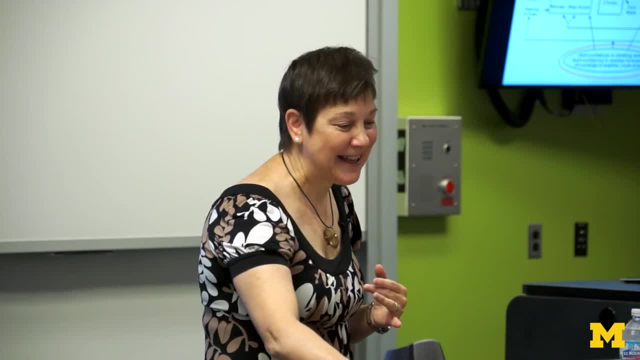 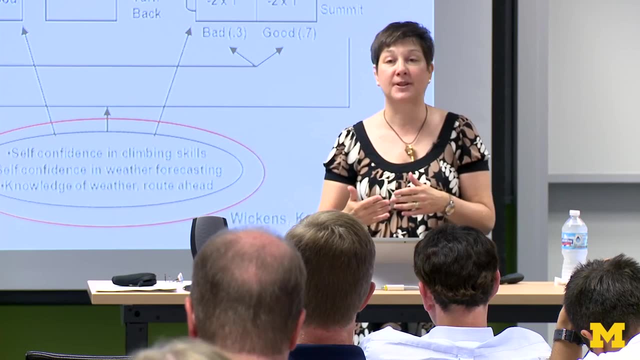 good idea, all right. and then there are other things that are going to influence this, which is: how confident are you in your, in your climbing skills, right? how much do you know about the weather personally? how much do you trust the information that you have? so what Chris was trying, 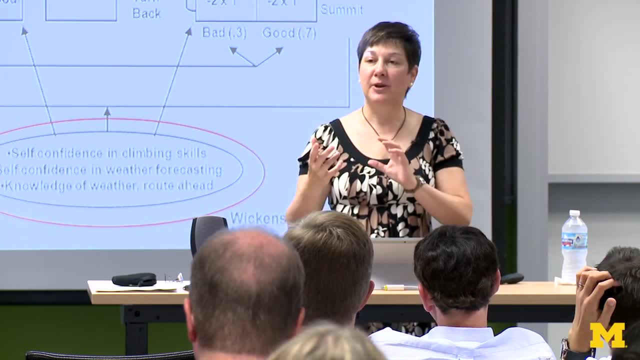 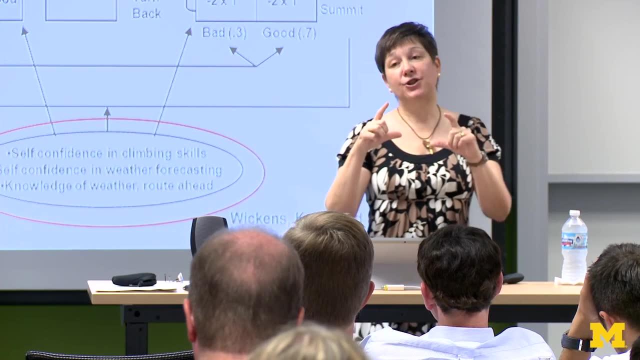 to do. Chris Wickens, in putting this model together, was trying to take what we know about the information processing structure and other factors that influence decisions. so, as you think about supporting decision-making, you want to be thinking about all these different features that play a role in. 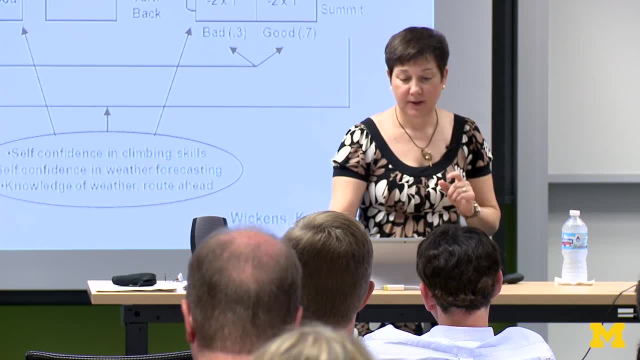 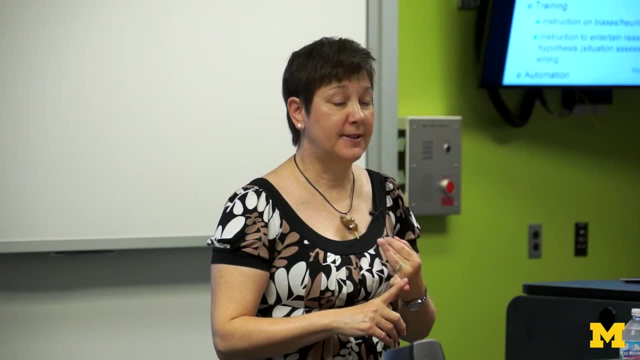 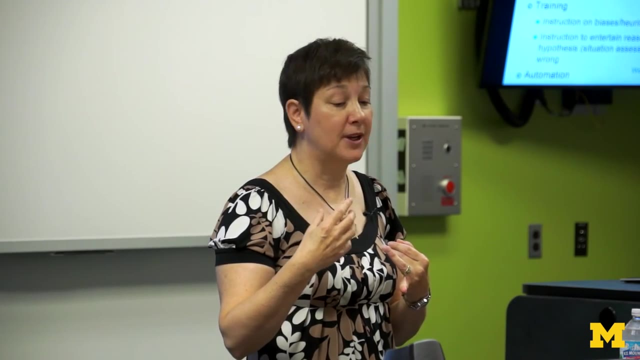 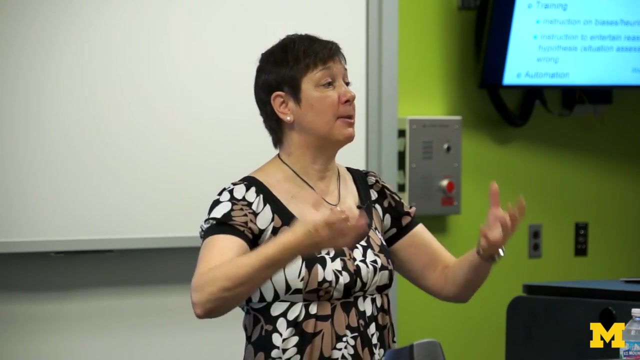 decision-making. all right, so you can use display technology to help support the decision-making process. so if you know that certain cues are likely to be less perceived, you can either make them all equally perceptually available or you can make the more diagnostic cues more salient- right, you can actually make them pop out in some way. you can also rely on